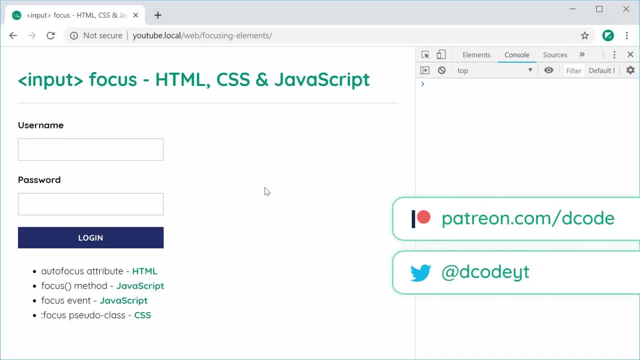 Hey guys, hey going. my name is Dom and in this video I want to shed some light on what it means to focus an input field. So for those of you who don't know, essentially focusing an input field looks like this: If I was to click inside this username field, this field. 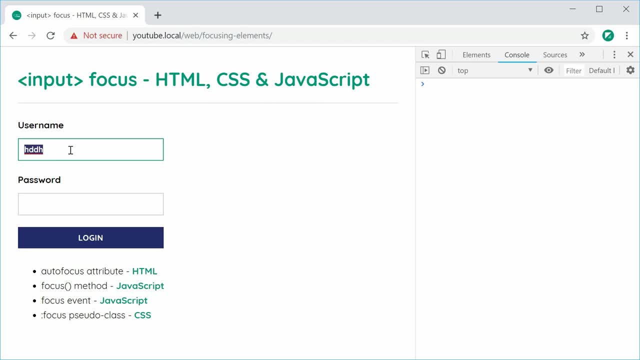 is now focused. I can start typing inside it. we can see the text cursor or prompt is flashing and the outline changes. So now this field is focused. this field is not, So the opposite of this is known as blur. So right now, both these fields are unfocused. 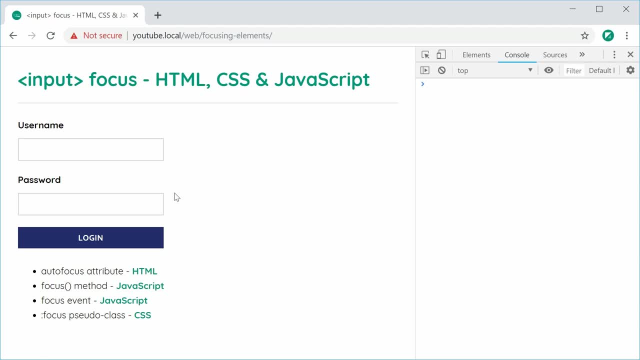 and, in other words, they have been blurred. So I think the aspect or the concept of focus is very important when it comes to web development in general. So here we have this video covering various aspects of how to actually interact with, I guess, the feature of focus using HTML, Javascript and CSS. So we're going. 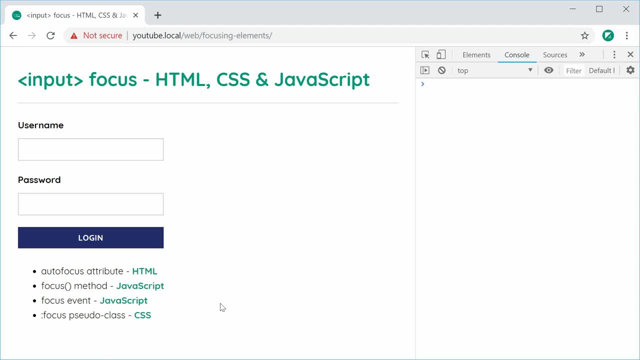 to cover all these four things inside this video. So let's begin with the autofocus attribute. So, essentially, this one allows you to automatically bring focus to an input field when a page or when the page loads up. So right now, if I was to refresh this page, we can see that. 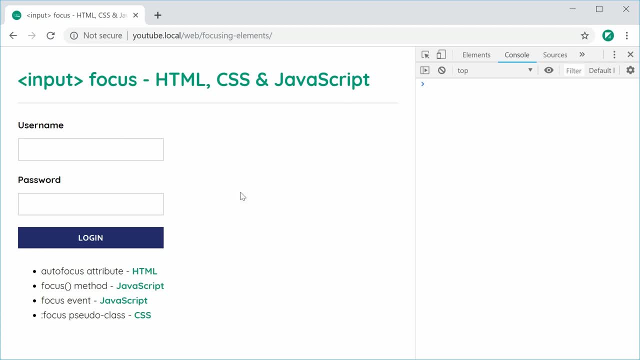 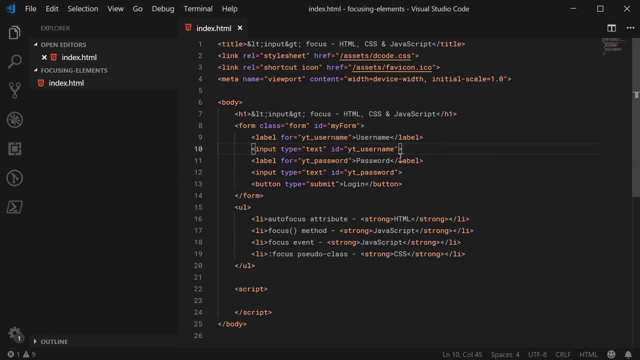 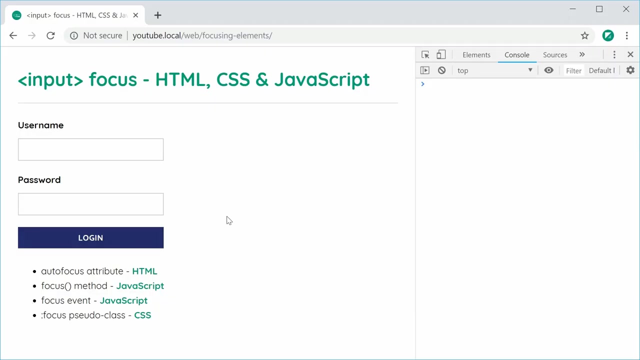 none of these input fields are focused. So I can go inside. I can go inside the HTML and then I can go inside, for example, the username input field, and I can add the autofocus attribute, just like that. I can now save this and refresh the browser and now we can see that the field has been focused automatically when the page. 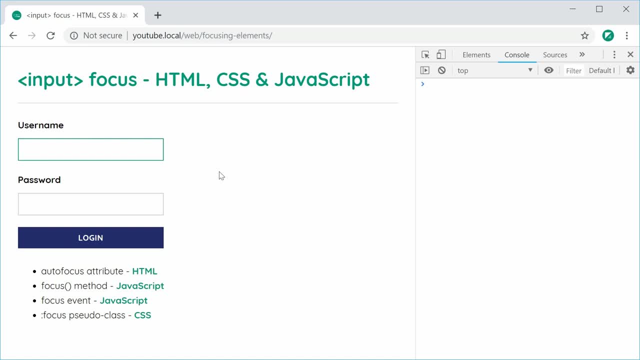 loads up. So this right here, I think, is pretty much essential for any sort of login form, because then your user can conveniently start typing in the username straight away without any other form of interaction. Okay, so that right. there is the autofocus attribute in HTML. We can now move on to the 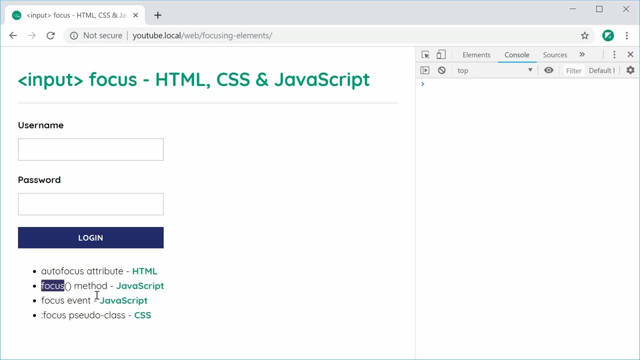 focus method, which is found in Javascript, and this one right here, allows you to manually force focus on a particular input field using Javascript. So, for example, here to demonstrate, I'm going to wait until the page loads up again and then, after three seconds, I want to bring focus to the password field. 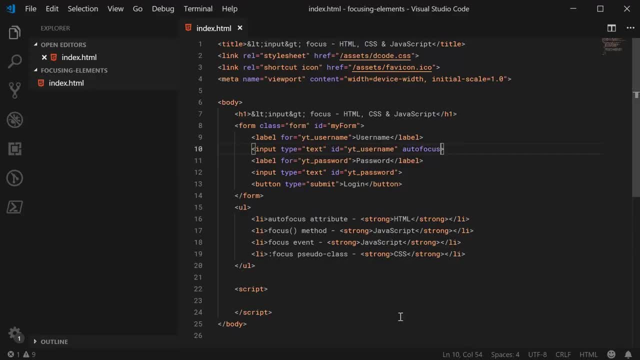 Okay, so let's go inside the text editor and remove the autofocus attribute from the username field and go inside the Javascript, and first we need a reference to the password field itself, because you're going to call the focus method or function on the actual field itself. 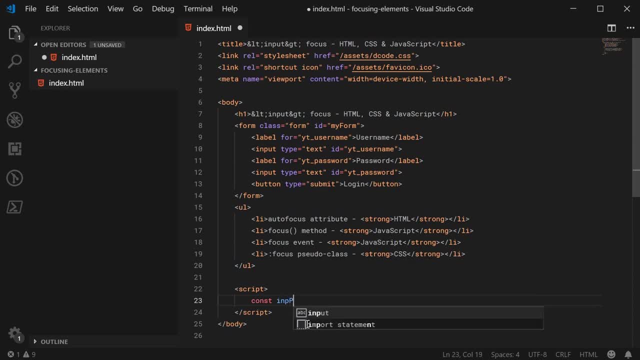 So let's make a new constant Call this one impPassword equal to documentjavascript. Okay, So documentgetElementById. I'm going to pass inside here yt underscore password to of course match the ID on the password field. I might just change this to type password. 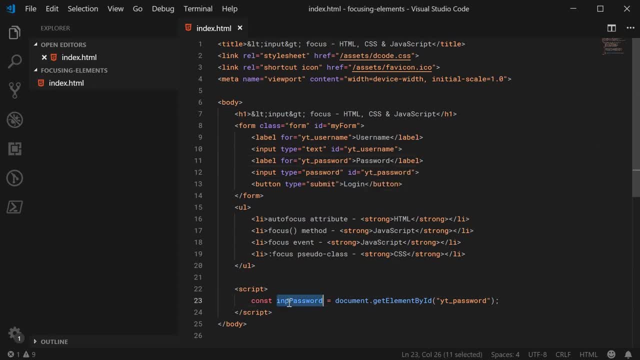 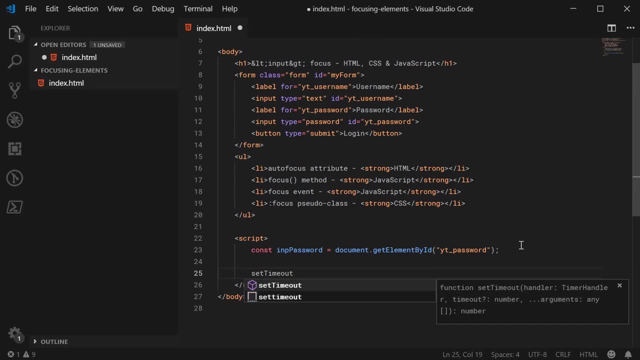 Okay, Cool. So now we have the impPassword reference in Javascript, We can simply use a setTimeout here and say after three seconds. so I'll just put a function inside here. So I'm just going to say after three seconds and we're going to say impPasswordfocus. 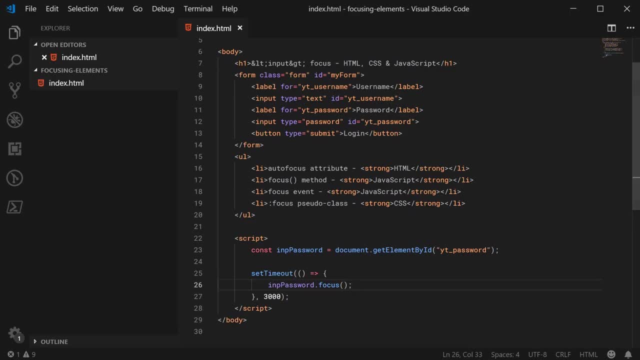 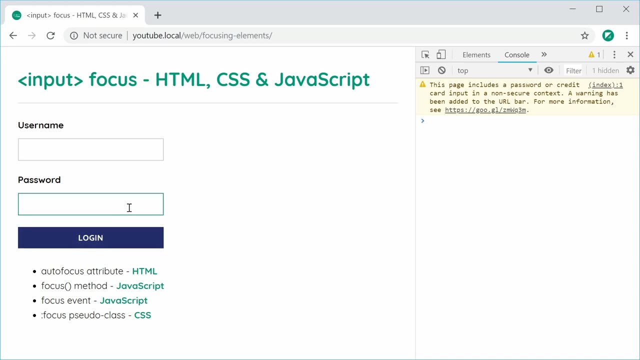 Okay, so it's simple as that. I can now save this and then refresh the browser and then wait three seconds, and we can see here that the password field now has focus. So you can, of course, maybe do things such as have different panels on your website. 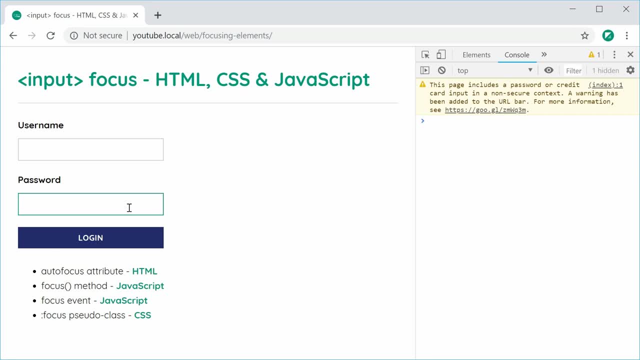 You know, when you open a new panel, maybe an input field inside there. So that is the focus method. with Javascript We also have the focus event. So essentially this means you're able to react to when your user brings focus to an input field. 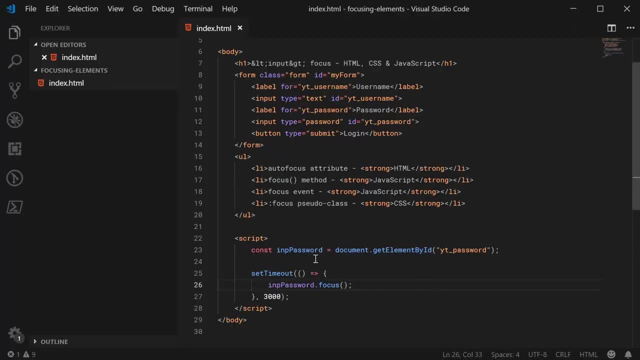 Okay, So let's go back inside here and take a look at that. So we're going to use the impPassword field once again. We'll just remove the setTimeout from down here and we're going to say impPasswordaddEventList. Okay, 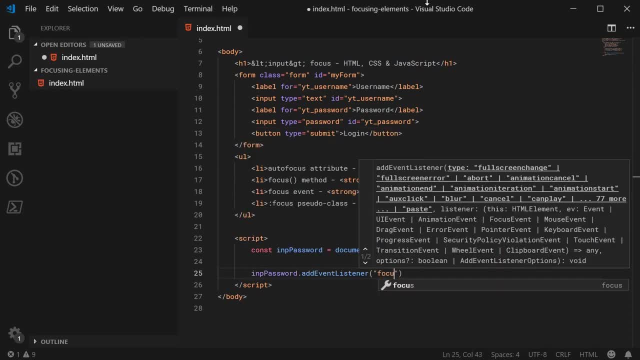 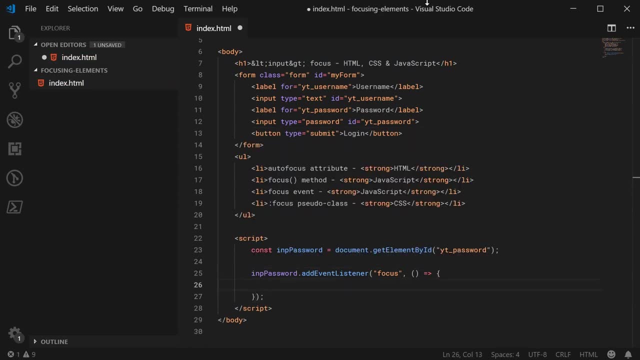 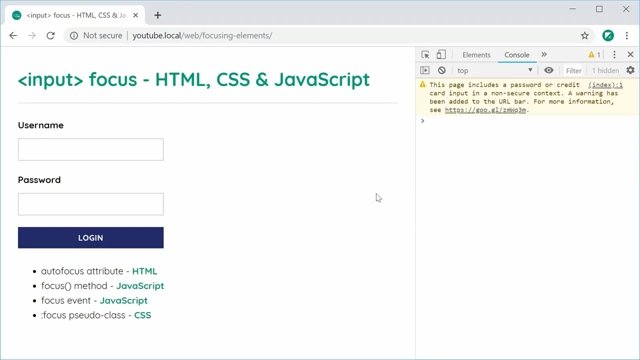 Cool, So we're going to put focus inside here And then for the callback function or the listener function, we're going to simply say consolelog, password field has focus. Okay, So pretty straightforward. Now, if I was to save this and refresh and click on the password field, we can see here: 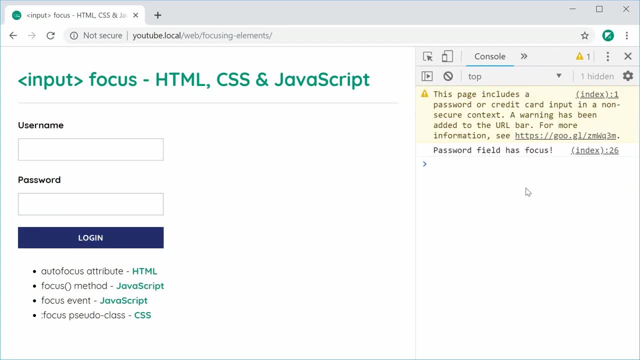 it says password has focused. So I'm going to click on the password field and we're going to see that it's focused inside the developer console. Okay, So that is the focus event in Javascript. I'm not sure why you'd want to use this, but of course, maybe you want to display some text. 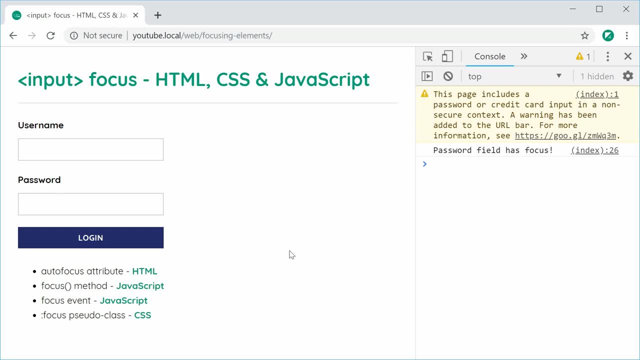 once the user clicks on a field, such as the requirements of the field or any sort of hint about the field itself. Okay, Cool. So now we have the focus pseudoclass, which is found in CSS, and, of course, this is about styling your input field. 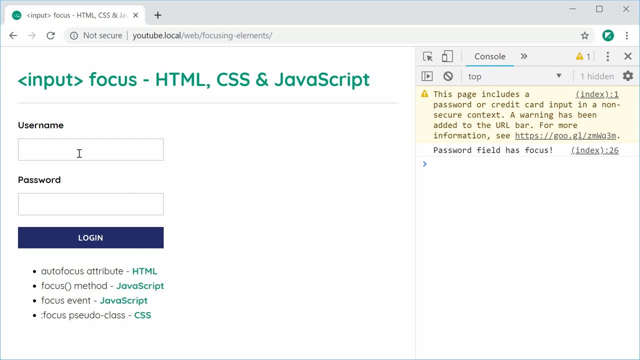 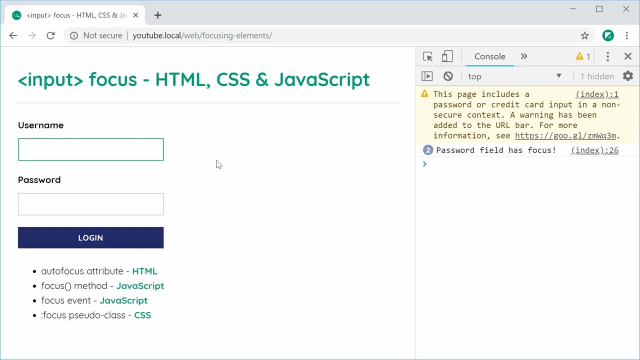 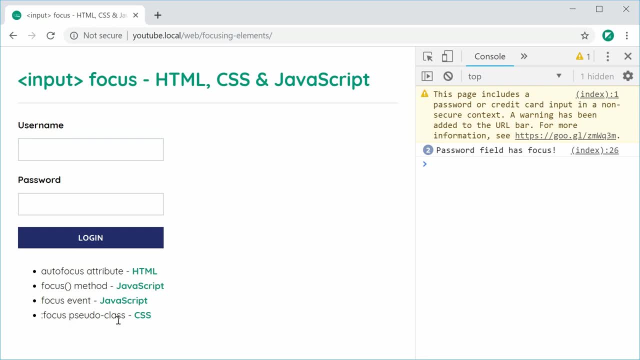 styling your input fields. So now we have the focus pseudoclass, which is found in CSS, and of course, this is about styling your input fields. So I've actually got one happening right now on these fields. but to demonstrate, let's go inside the style tag of this document, which I'll now create. 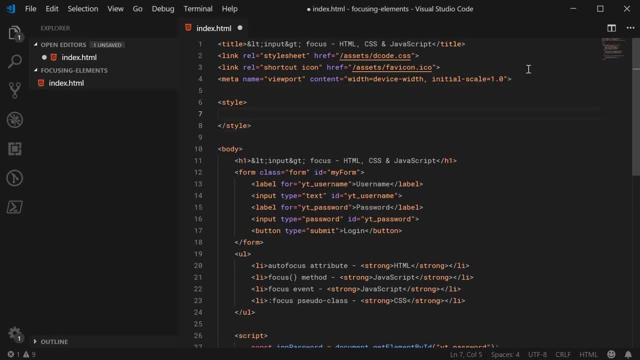 So let's make some CSS rules And I'm just going to say here, for each input, seria field. so I'll say I'll just actually target the form class, so this form, right here, and say form and then input for each input. you know what I've got to add: the focus, pseudo class, the most. 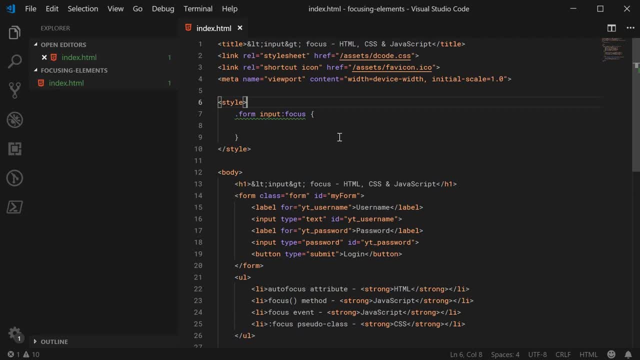 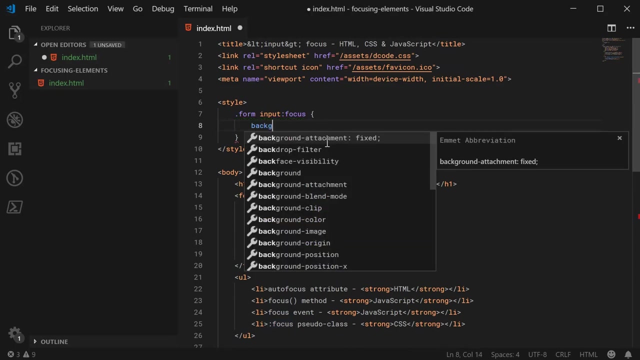 important part about this, this segment, I guess. so here we're saying: when a input field inside the form has focus, okay, so that's the pseudo class right there, we're going to change things about it. so, for example, let's just say we can say background and then red, okay, so pretty clear.